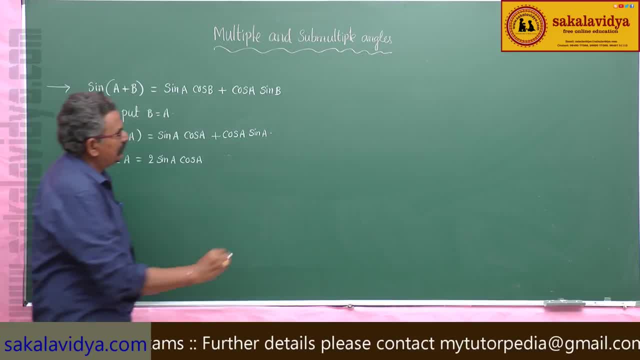 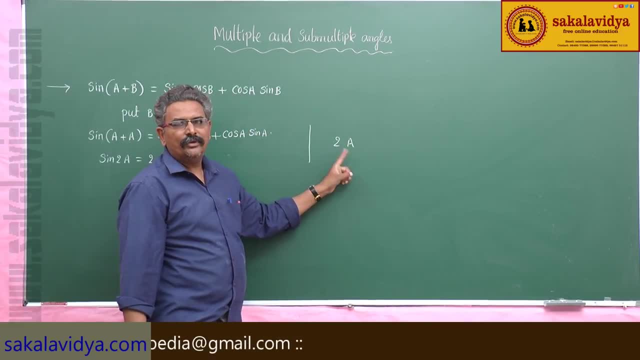 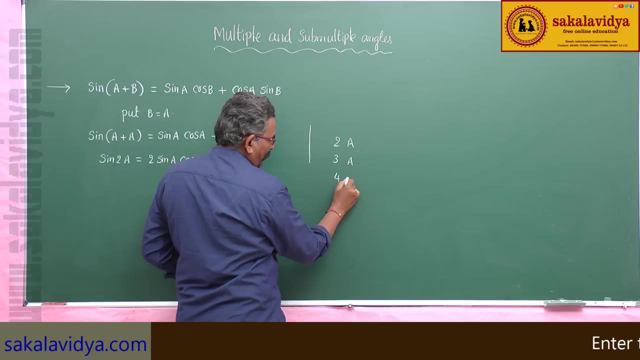 now here just observe 2 a. So now this 2 a is the multiple of actually a is the multiple of 2.. Similarly we get 3 a, 4 a, 5 a, and like that We will get it 3 a, 4 a, 5 a, and so on. We can. 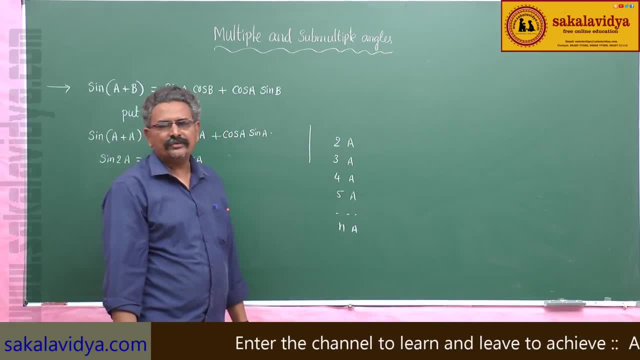 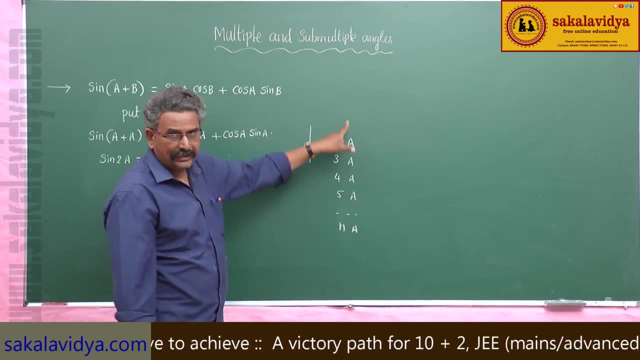 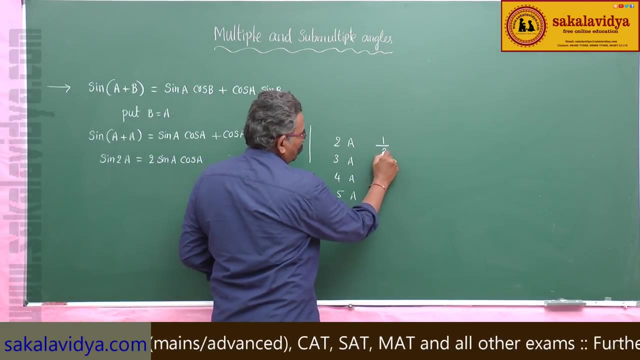 write a where n is a n positive integer or it may be negative integer. n is a integer, Then this is the multiple angles. Similarly, if angle a are the multiples of 1 by 2,, 1 by 3,, 1 by 4, and so on, 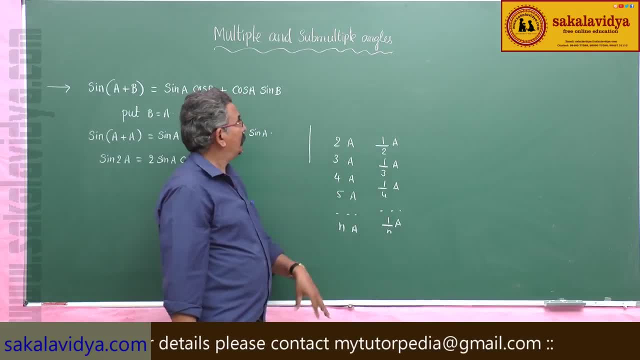 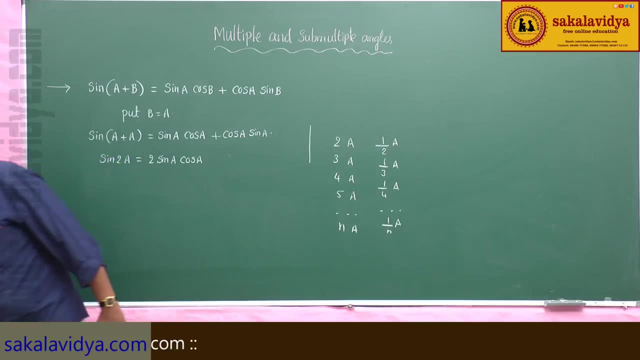 1 by n of a. These angles are called submultiple angles. We shall discuss the submultiple angles later. First we shall go in detail about the multiple angles and their formulae. That means the prospective formulae. Now the first formula is: sin 2. a is equal to 2, sin a, cos a. 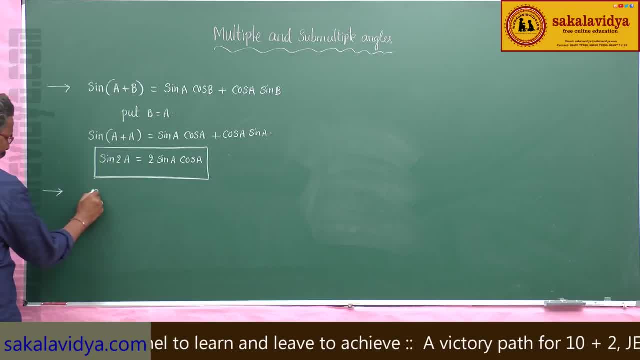 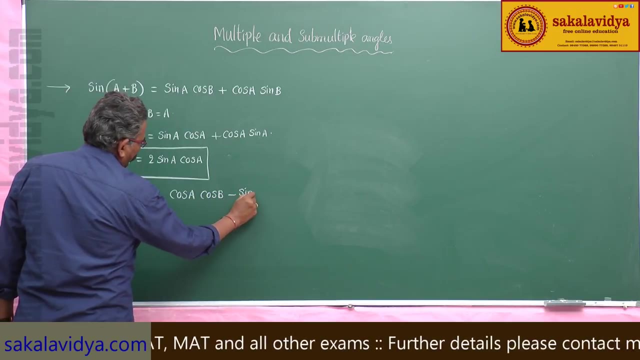 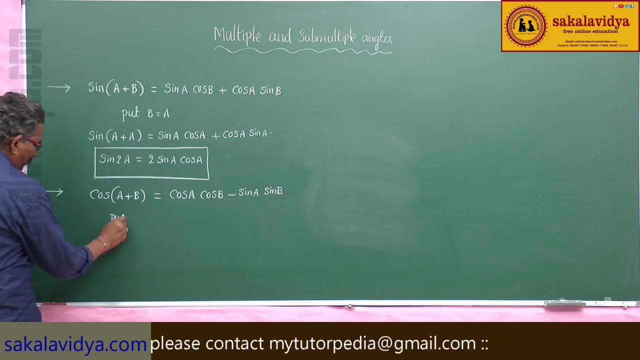 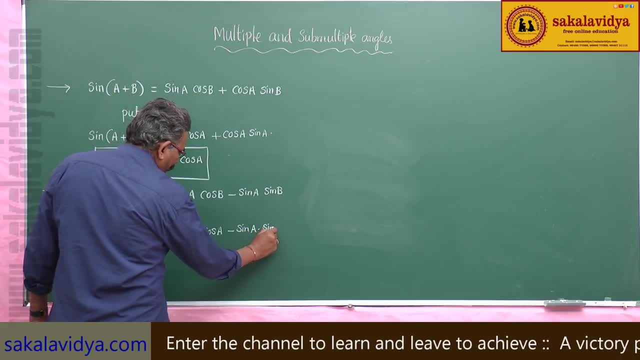 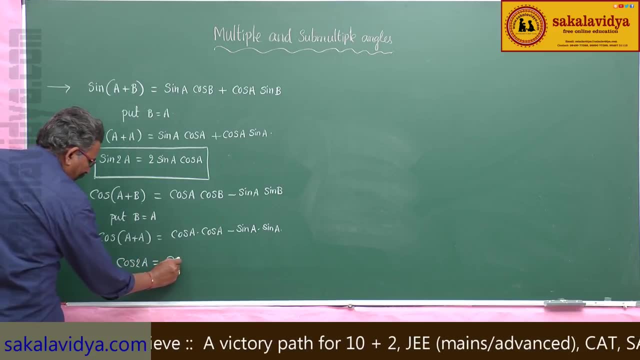 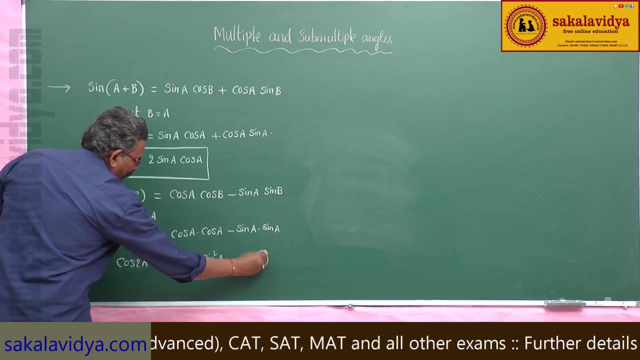 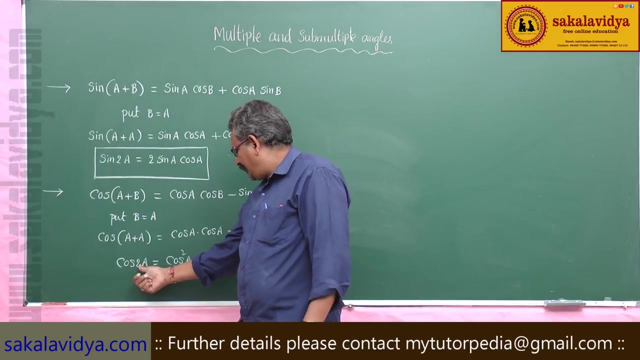 sin a into sin a. now, this is cos to a, equals to cos a into. cos a cos square a minus sin square a, say this is equation 1.. Now so let us suppose can we change this cos to a in terms of cos a, and also can we change this cos to a in terms of sin a into. 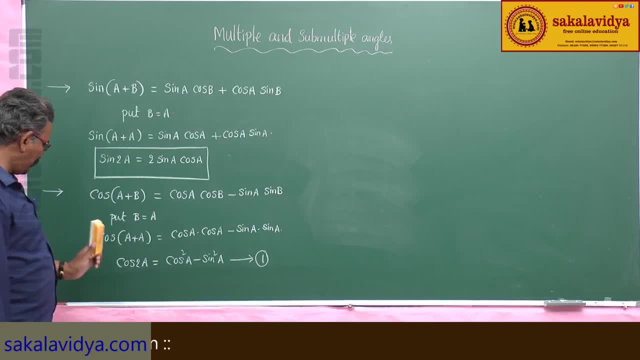 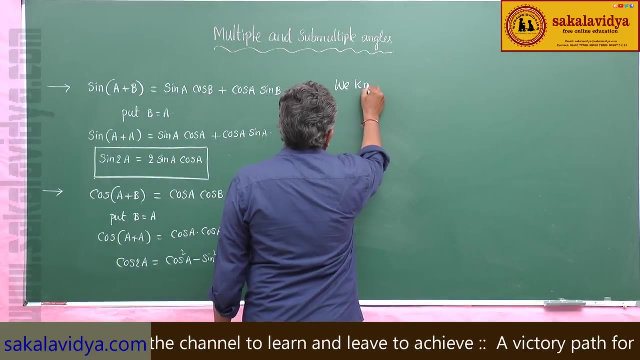 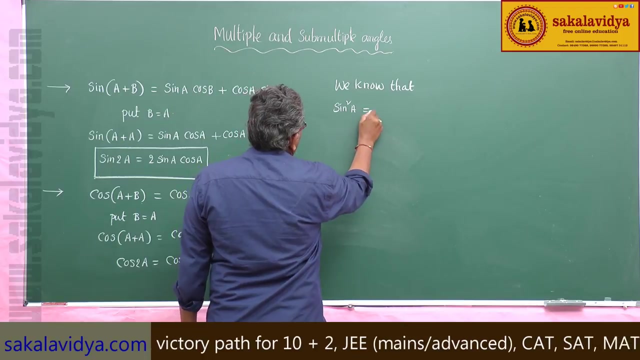 cos a. First, let us change this cos to a in terms of cos. so that means now we have to change sin square a in terms of cos square a, since we know that. we know that sin square a equals to 1 minus cos square a. 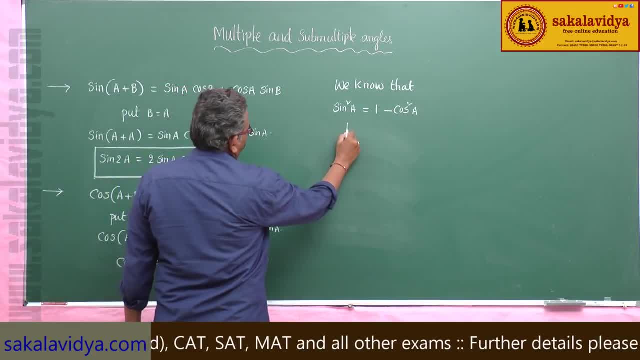 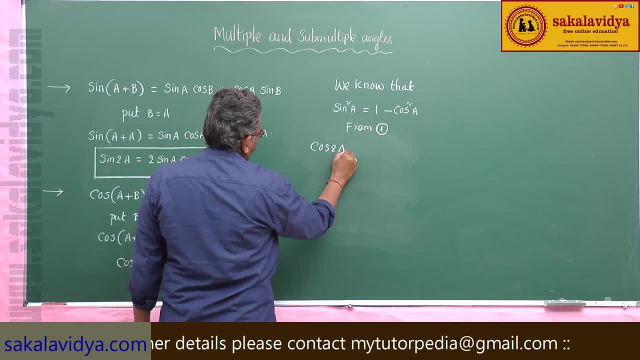 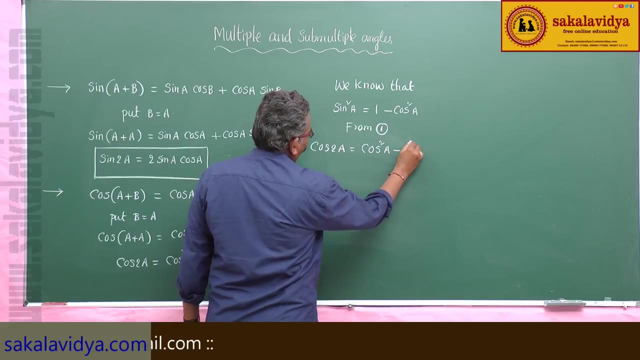 Now from 1.. 1.. 1. this cos 2a we can write from 1, this cos 2a we can write cos square a and minus of 1 minus cos square a. this is cos square a and minus 1 plus cos square a. 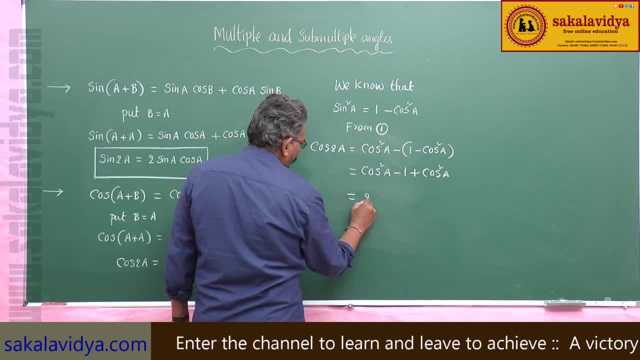 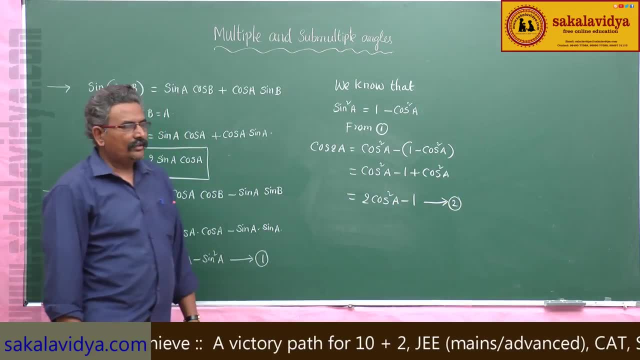 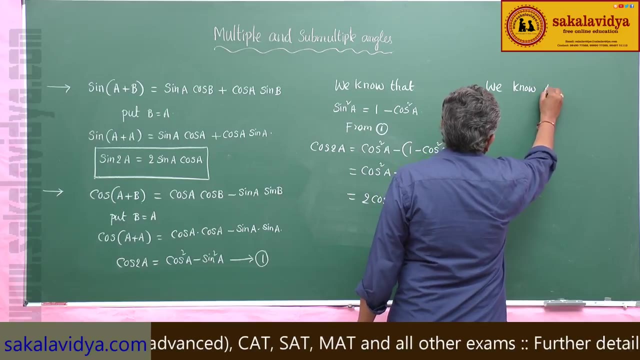 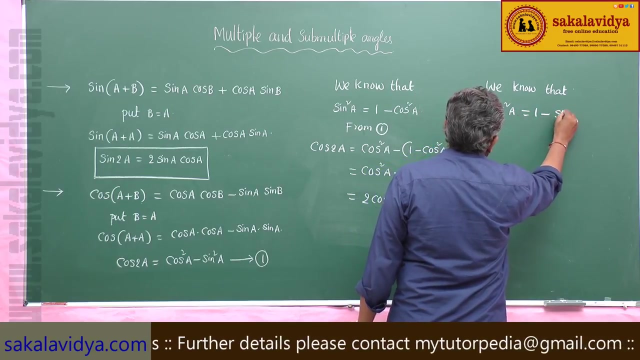 So this is 2. cos square a and minus 1 say this is equation 2.. Now we know that this cos square a is equal to 1 minus sin. square a again from 1. it is the elite square from 1 to 1 minus sin pa. 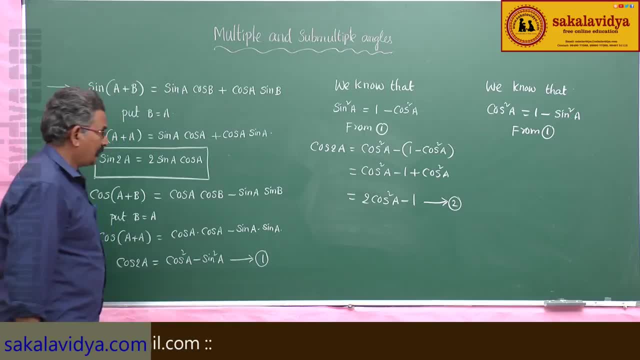 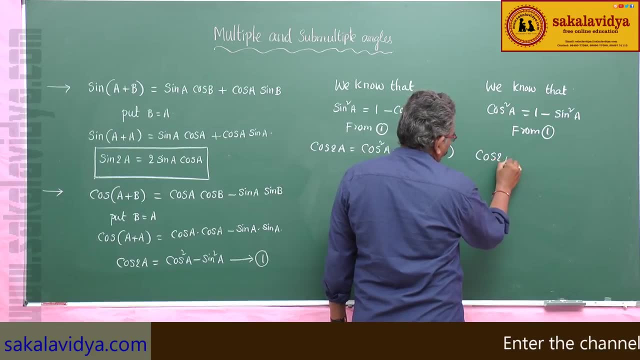 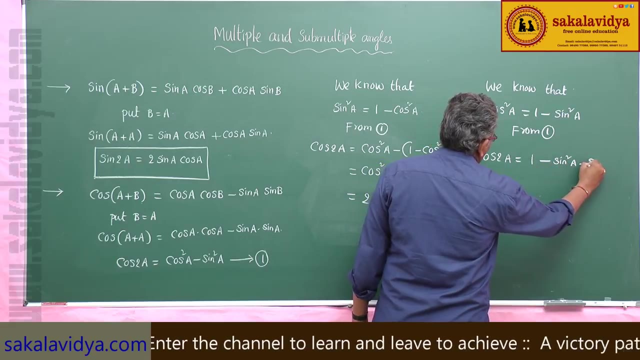 1, 2, cos red wave a, Because did not call sin square a from 1.. So this equation, this cos square, is replaced by 1 minus sin square a. So cos 2a value can have like this: 1 minus sin square a and minus sin square a. So we have 1 minus. 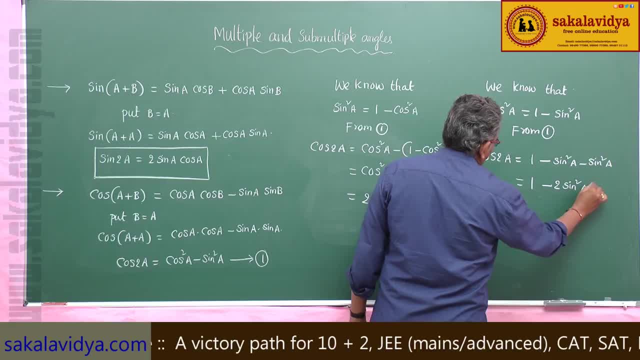 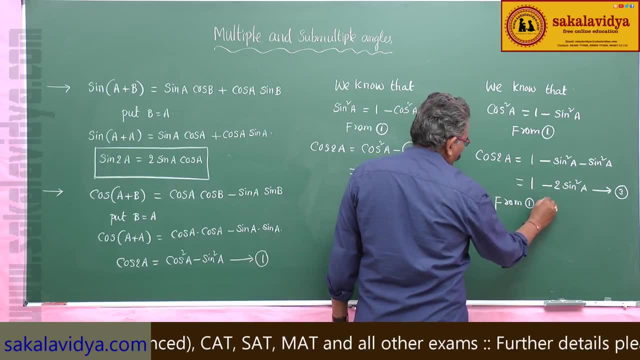 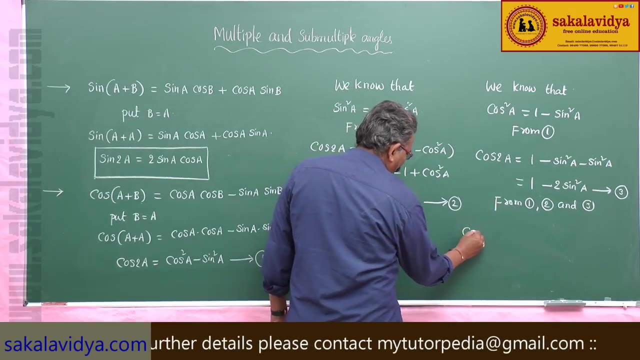 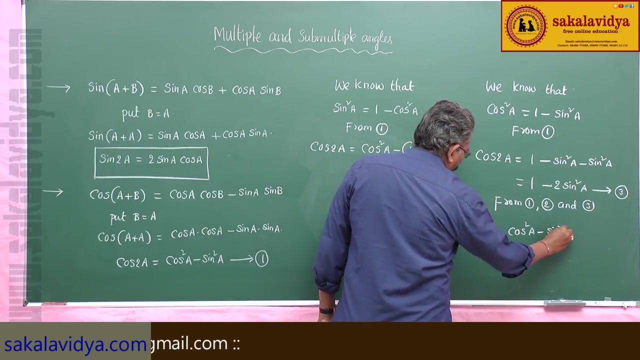 2 sin square a. This is equation 3.. So from 1, 2 and 3. So cos 2a can be stated as cos square a minus sin square a. 2 cos square a minus sin square a. 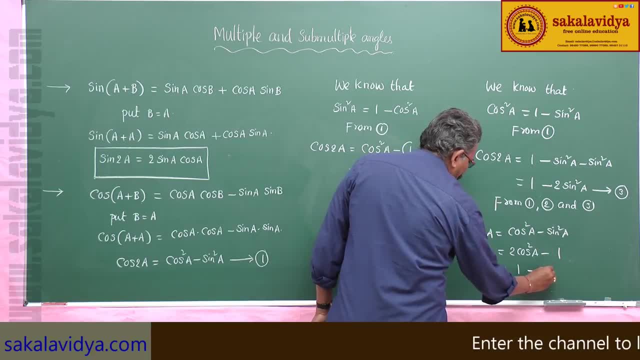 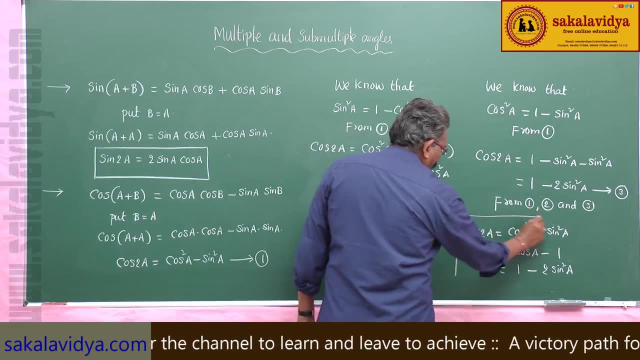 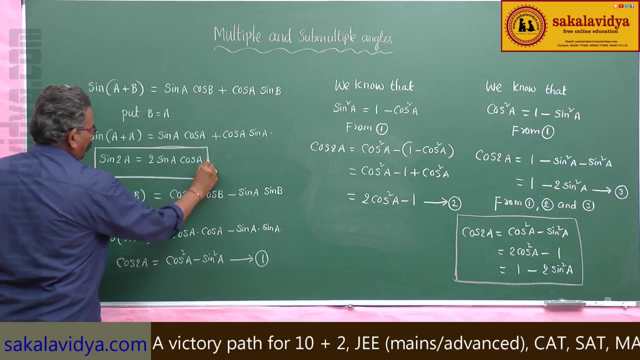 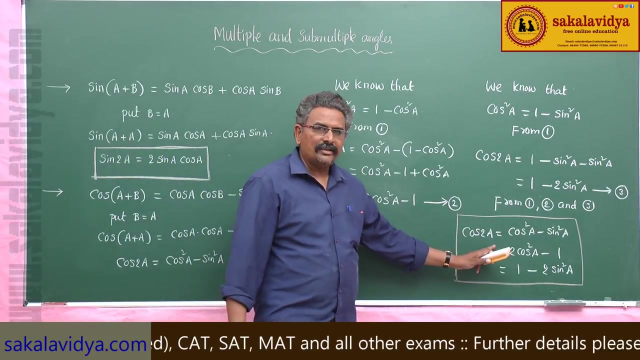 minus 1, or 1 minus 2 sin square a. So these now, let me repeat once again: sin 2a is equal to 2, sin a cos a, and whereas cos 2a is equal to cos square a minus sin square a or 2 cos. 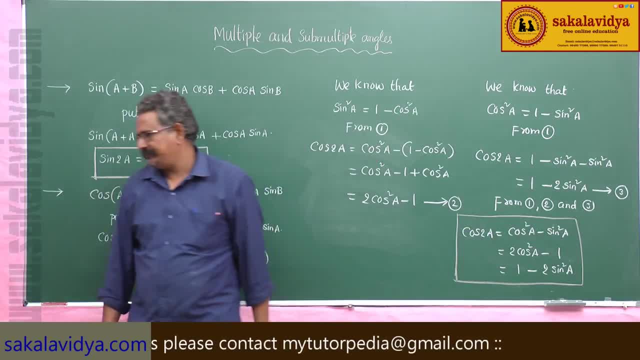 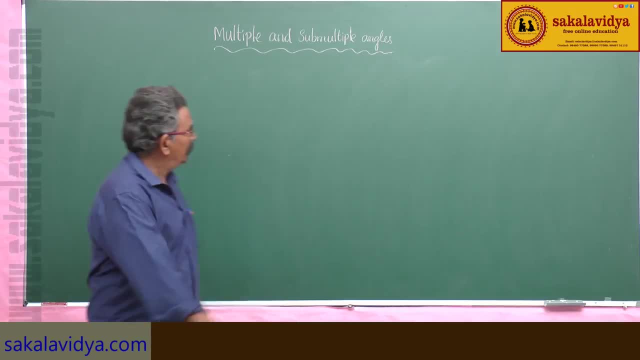 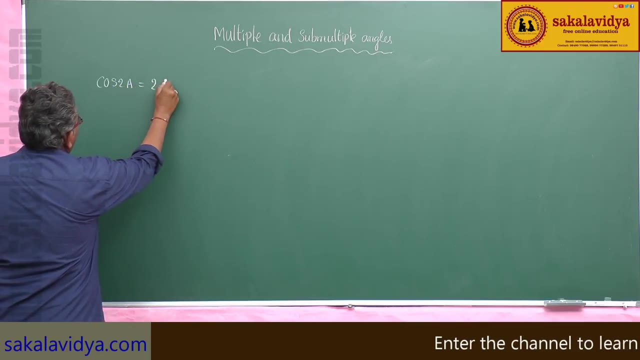 square a minus 1 or 1 minus 2 sin square a. We know that cos 2a is equal to 2, cos square a minus 1.. Now bring minus 1 this side, So we get 2 cos square a is equal to 1 plus cos. 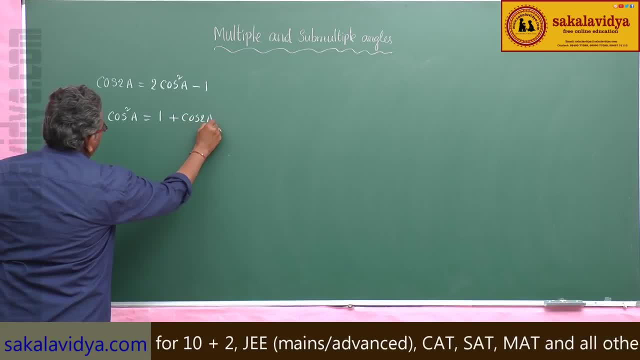 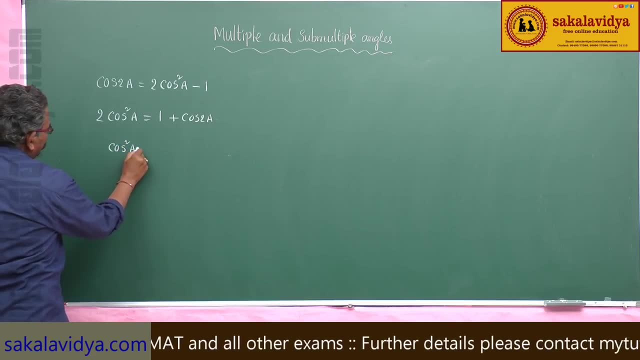 2a. That means 1 plus cos 2a is equal to 2 cos square a. Now cos square a is equal to: we can write 1 plus cos 2a by 2.. What is cos a? It is plus or minus root of 1 plus cos. 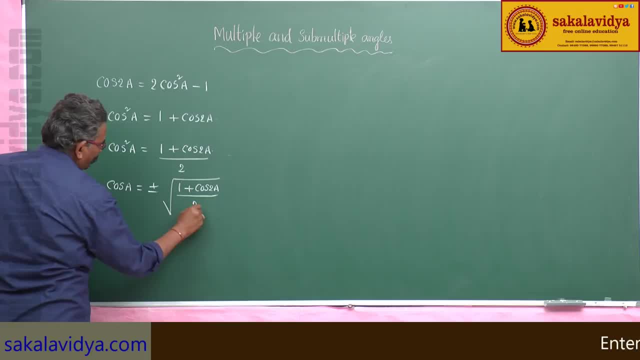 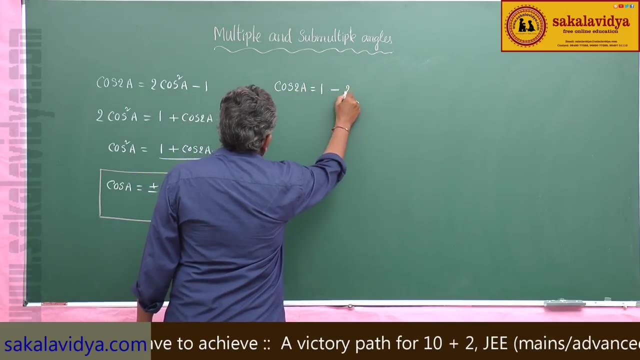 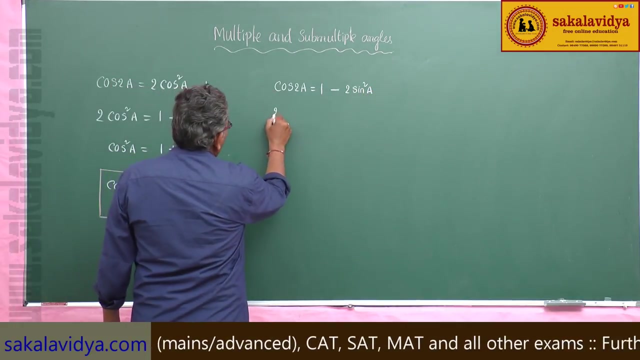 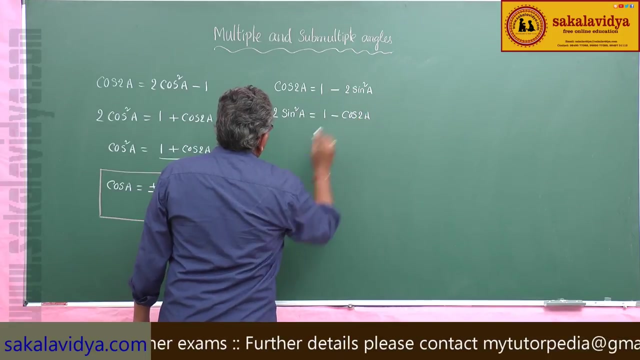 2a by 2.. So this formula, we get it. Similarly, we know that cos 2a is also 1 minus 2 sin square a. Bring minus 2 sin square a this side, So 2 sin square a equals to 1 minus cos 2a. So this sin square a is equal. 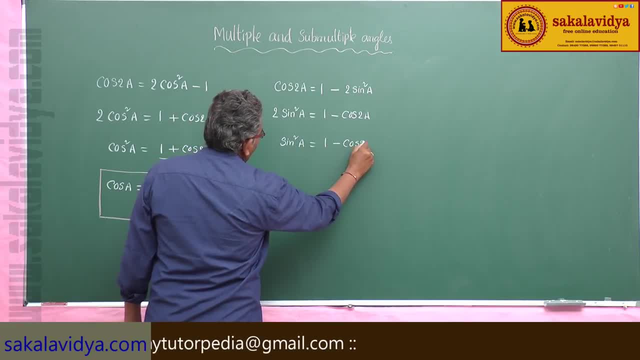 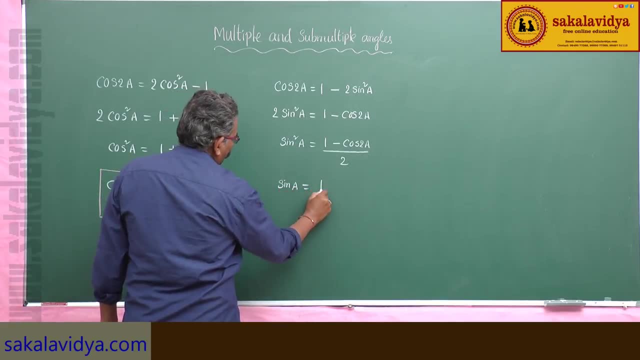 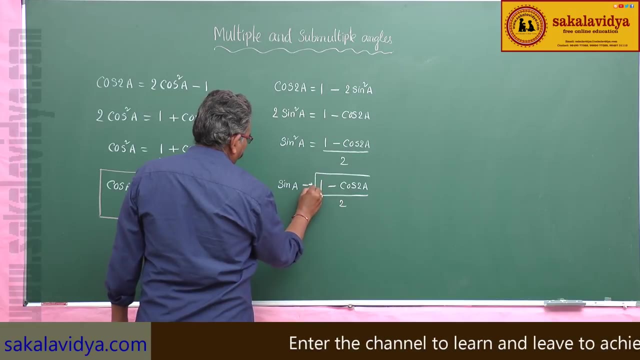 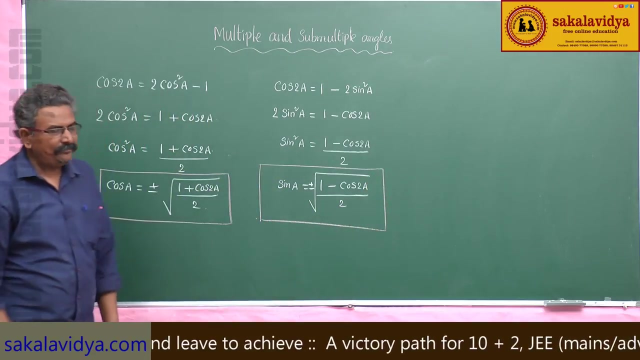 to 1 minus cos 2a by 2.. Now sin a is equal to 1 minus cos 2a by 2, root plus or minus. So now let me repeat once again: 2 cos square a means 1 plus cos 2a and cos a is: